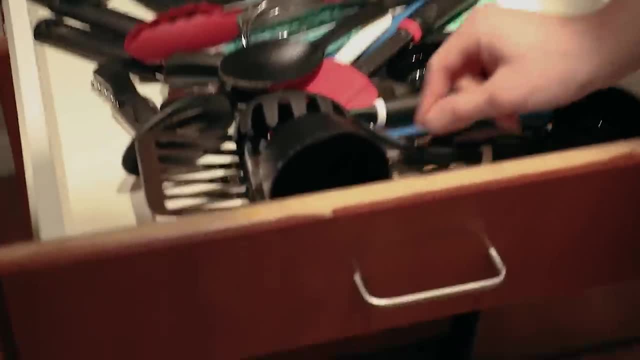 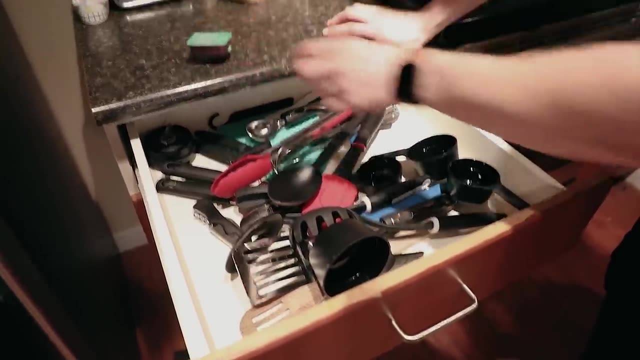 Not sure why that knife. That should not be. And notice how it's facing up. Yeah, Not my doing, Don't um? just a quick tip: Measuring cups, That's what good. There is a ranch in there. This is so sorry, Sriracha, Okay. 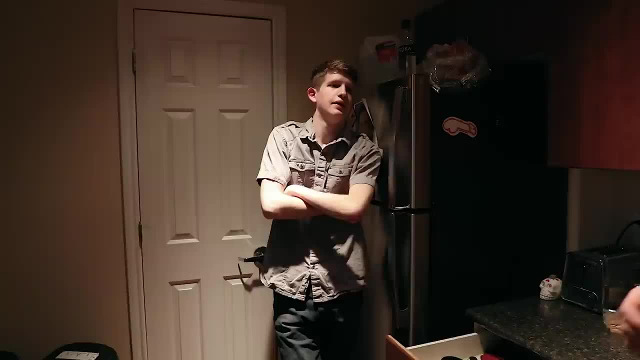 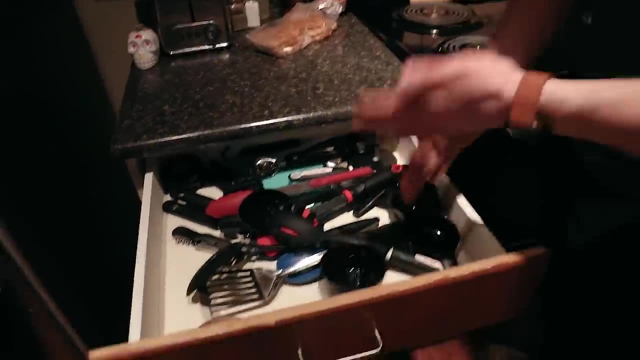 You can just put those in there. Yeah, In the cabinet It's still on the door. A little bit of a flour, Hopefully, Oh so basic pots, basic pans, No more, no less. I'm not going to include the walk Cause, I'm just 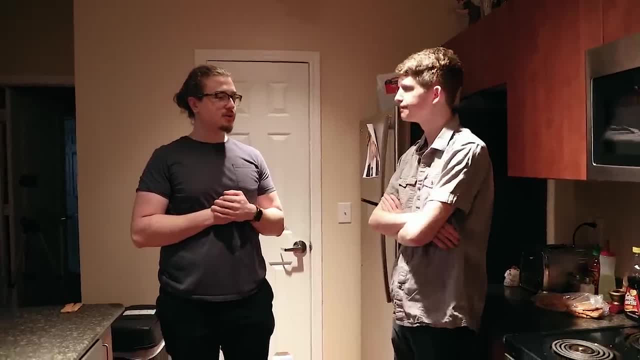 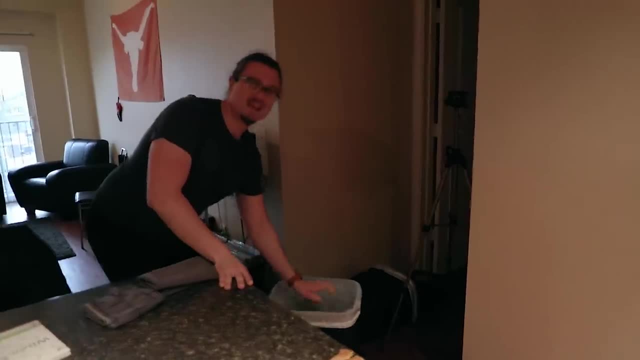 going to assume people don't have a walk. I feel like we're good. Yeah, I appreciate you letting me come in and uh, and and raise the place and I will make my exit, and Let me just put that in a better spot. 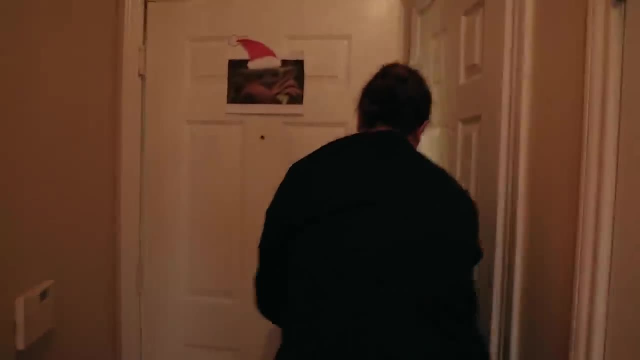 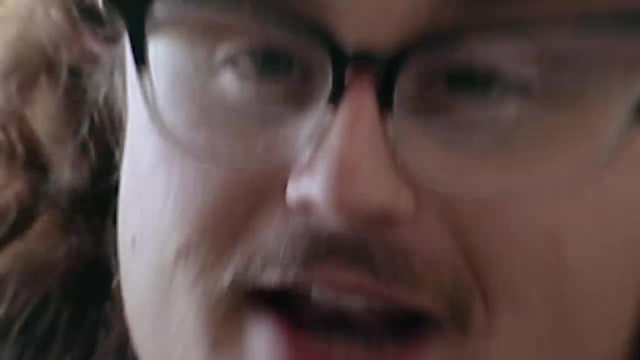 I just let's go, We're going to go, Thank you, Thank you so much. Nothing better than going into an innocent person's home, razzing them because the way that they organize their kitchen- nothing better than that, Am I right, folks? 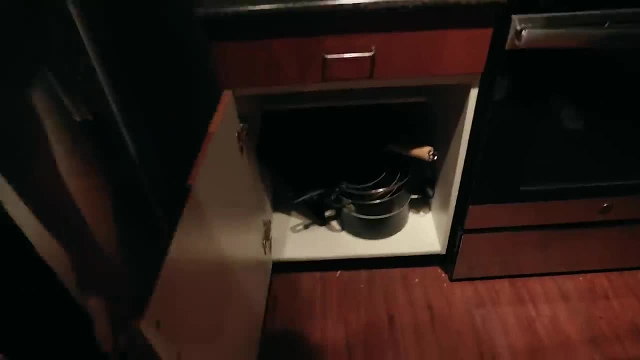 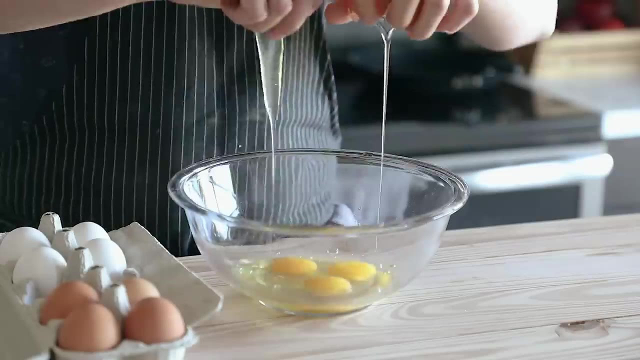 Based off of what they had. that's basically the parameters that I'm going to work with to develop these recipes. So, with all that said, let's do this, Shall we Okay. So the first one is going to be breakfast. This is essentially a leftovers for Tata. 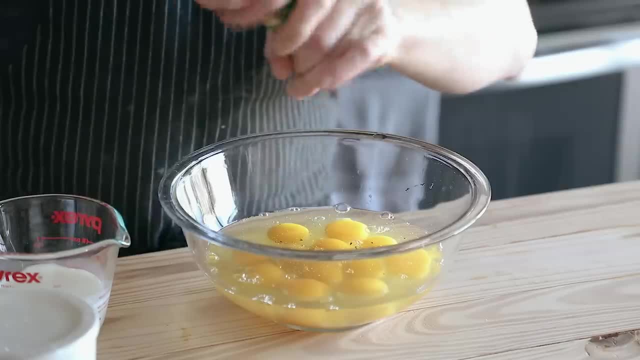 So you're going to need one dozen eggs, Yes, A whole thing, Half a cup or 120 milliliters of whole milk, salt and pepper to taste. Give it a little whiskey whisk And then in a 10 inch nonstick pan, 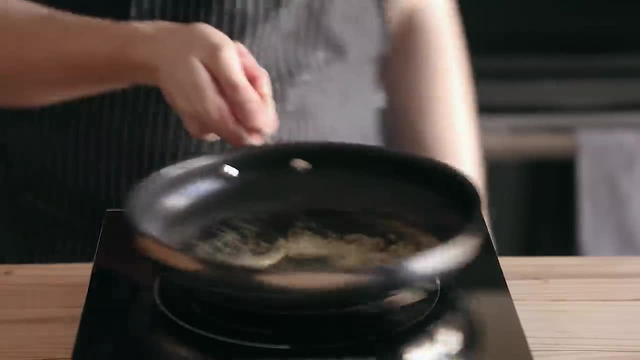 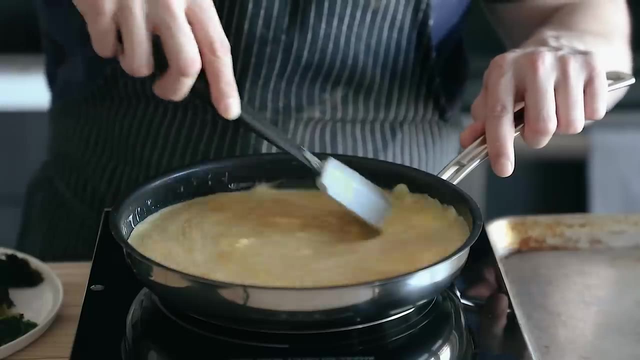 you're going to add two tail students or 24 grams of unsalted butter, Bring that up over medium heat until it's melty and boobily, pouring your eggs and then begin stirring and cooking. Now, once they begin to pull from the bottom, you're going to have one cup or 120 grams of. 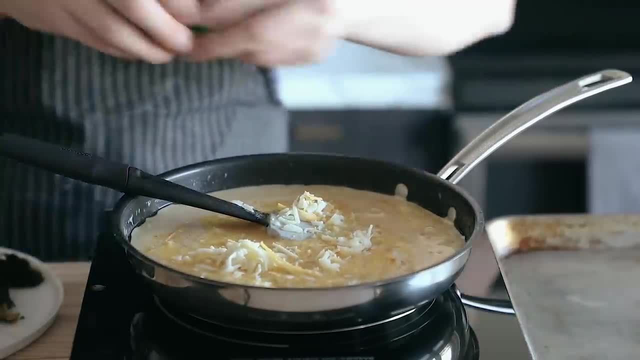 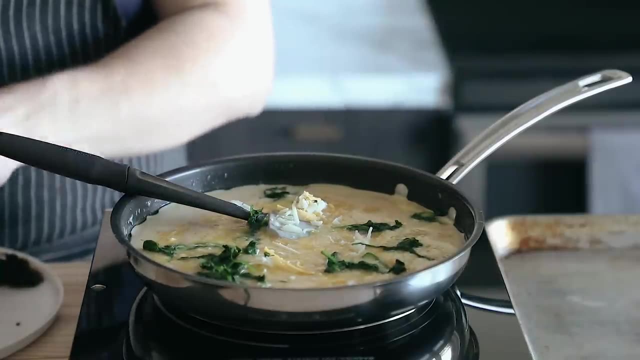 grade cheese. I did a couple of different ones: Menchego cheddar, you know you name- about a cup and about a cup and about a cup of cook vector and about a cup of cooked vegetables of your choice. Got it. Mix of spinach and broccoli, You know you do whatever you want. Mix until evenly distributed. 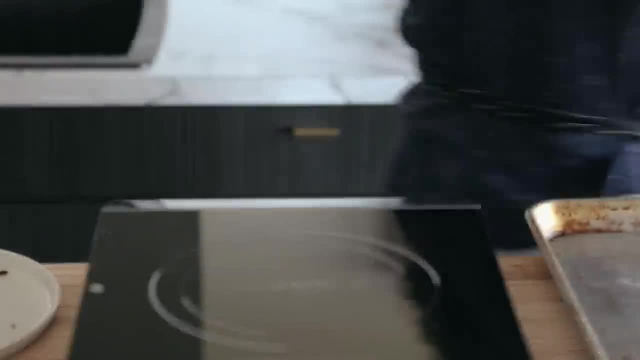 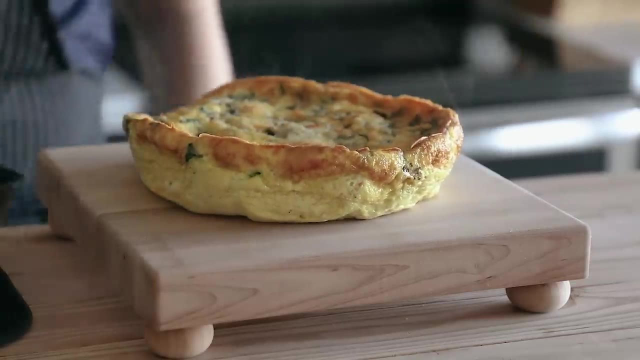 and then place it into it, and then place it into an oven preheated to 350 degrees Fahrenheit for about 25 minutes or until it looks like this. Look at that, This is a thick frittata. Now just let that cool to room temperature or you can serve hot. It's up to you. You do serve food. 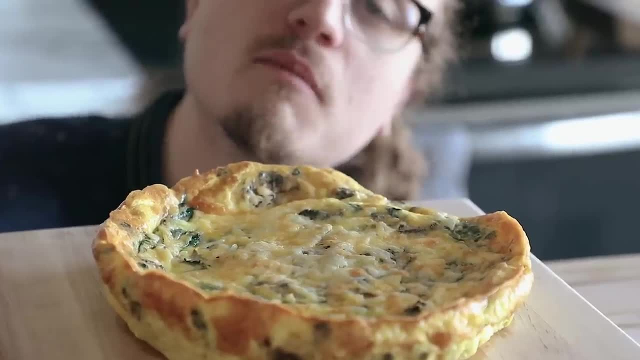 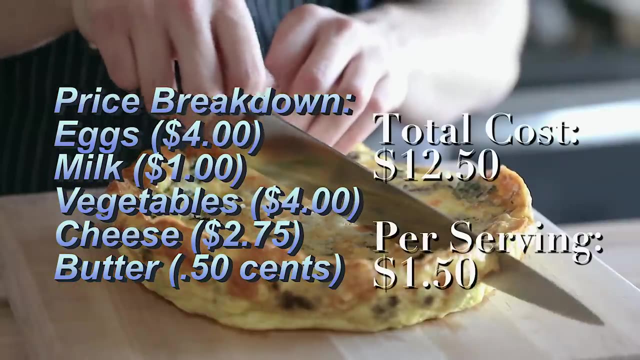 like that to people. Do you really think that I, do you think that I'm doing this in a serious way? The answer is no. Now here's a little price breakdown for you. This was the total cost at $12 and 50 cents, So that means that each serving is like a dollar 50. It's a good deal. 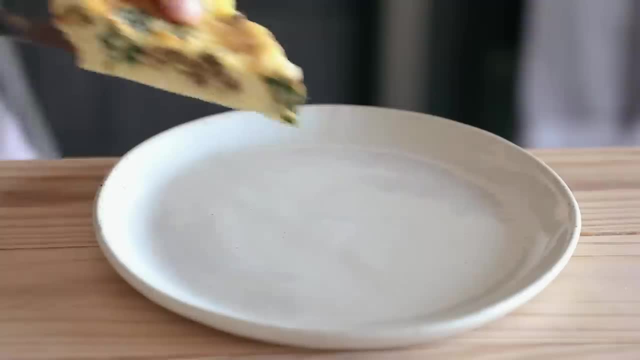 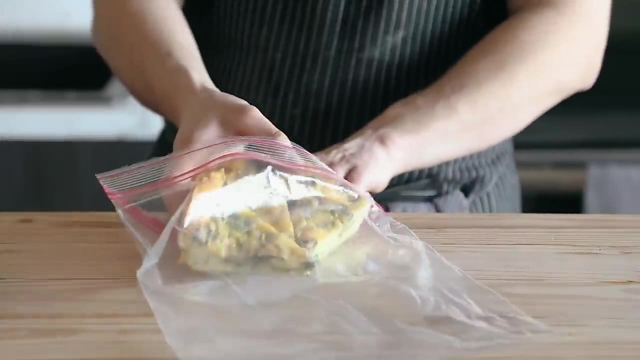 You can serve it room temp, You can serve it hot, You can serve it cold, as whatever floats your boat, There's nothing. there's no wrong way to serve it. really Serve it with maybe some avocado or some toast. Just go to town. This keeps really well in the fridge too. Tosses into a baggie or 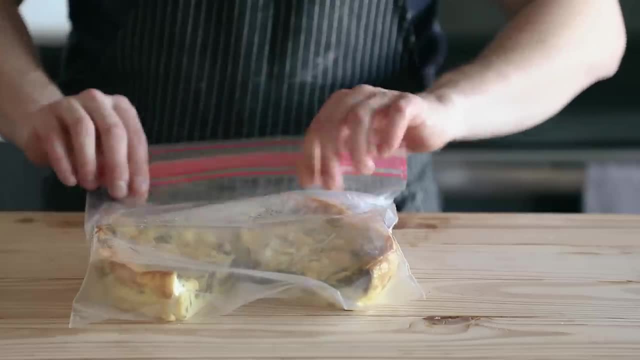 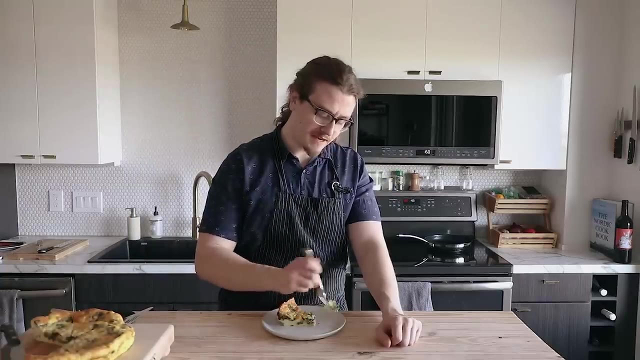 whatever storage container into your fridge and have ultra easy breakfast. Just make some toast, microwave one of these and you're good to go, Okay, So whoa, get out of here. Extremely easy to make Bag, take it with you to work. You see what I'm saying. This goes everywhere, This can. 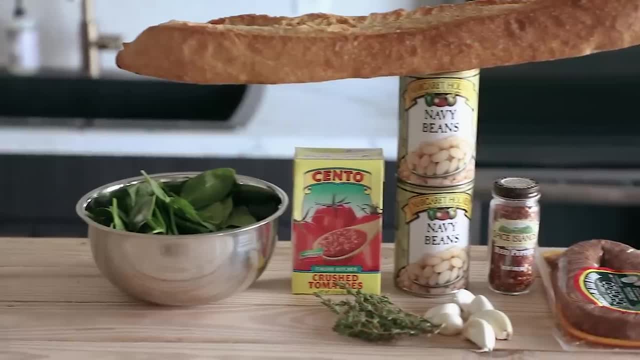 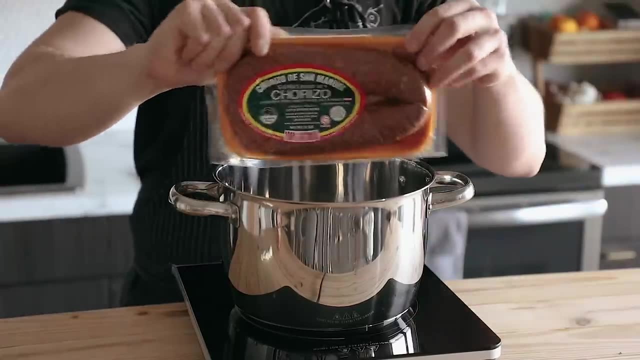 go everywhere. Well, not off the plate, though. Next up is the meal that I skipped eight times out of 10, lunch, And these are pretty much all the ingredients you're going to need, aside from some basics. In a medium sized pot, squeeze out a 12 ounce sausage link of chorizo. Yeah, You like. 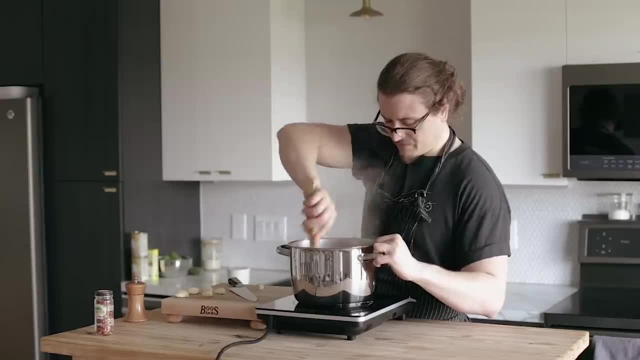 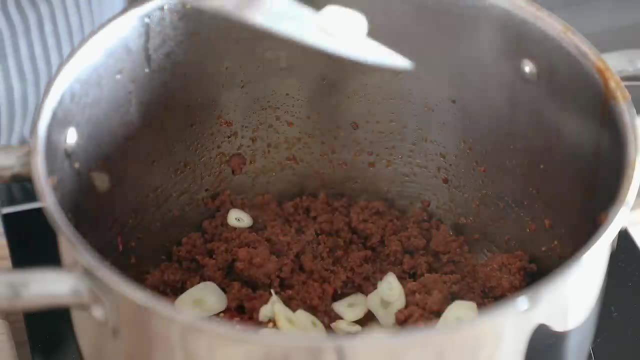 that, Yeah, Into the well, into the pot. Begin cooking that over medium heat until all the pork is cooked and you start to get some browning. Then you're going to add three quarters of a teaspoon or two grams of red pepper, spicy boys and four cloves of sliced garlic. Give that a little stir. 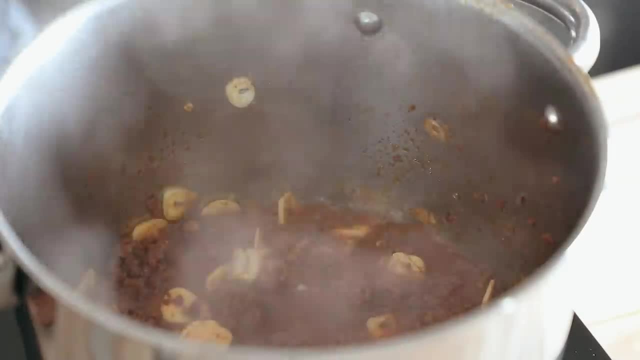 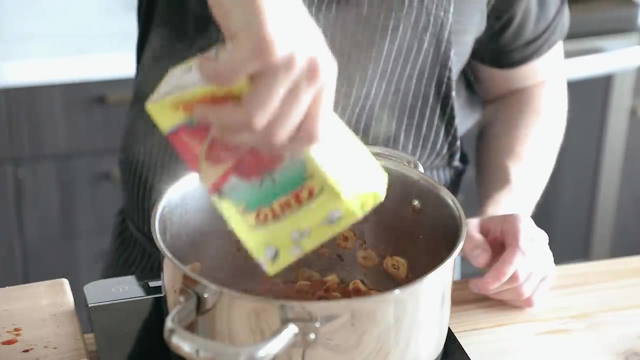 and continue cooking until fragrant. Then add half a cup or 120 milliliters of filtered water. Cook that down a little bit till it starts to look a little bit homogenous. Then add a 17.6 ounce or 500 gram carton of crushed tomatoes. Season that with a little bit of salt and pepper. 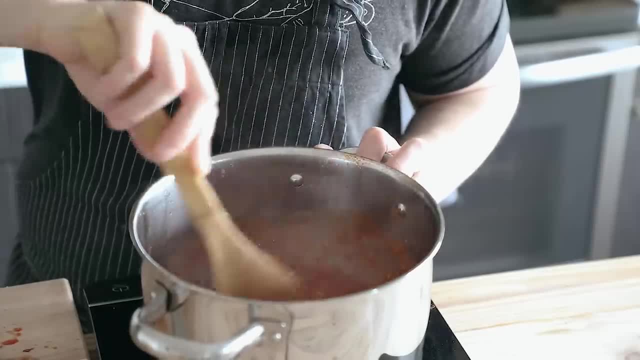 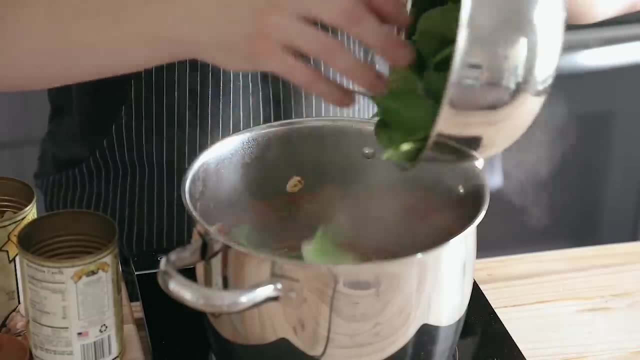 to taste, Give a little stir and let that simmer for 10 minutes. Oh, and, optionally, during that simmering process you could totally add a sprig of thyme or whatever herb you like. Okay, So once that's simmered- French people are having an aneurysm right now- You're going to add three. 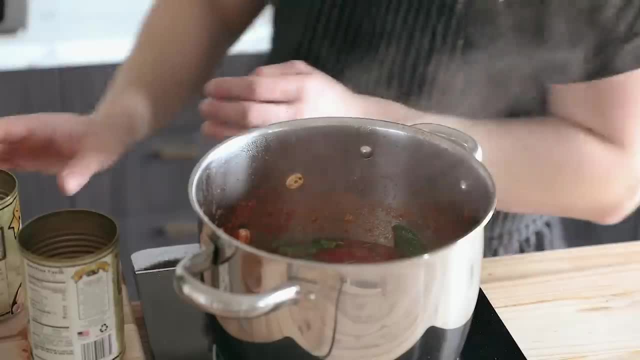 cups or 75 grams of baby spinach. Just let that sit in there until it wilts, followed by two cans of white Navy beans, And then you're just going to let that sit in there until everything's nice and heated through And that's it. That's the. 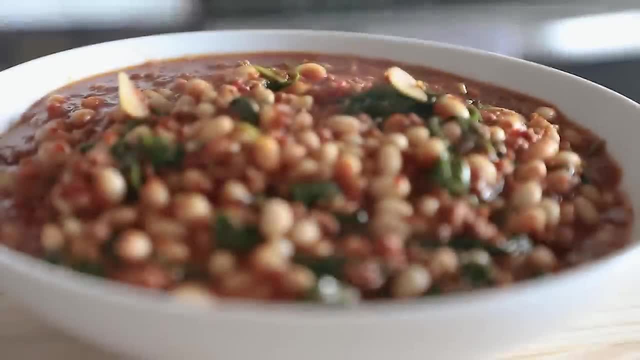 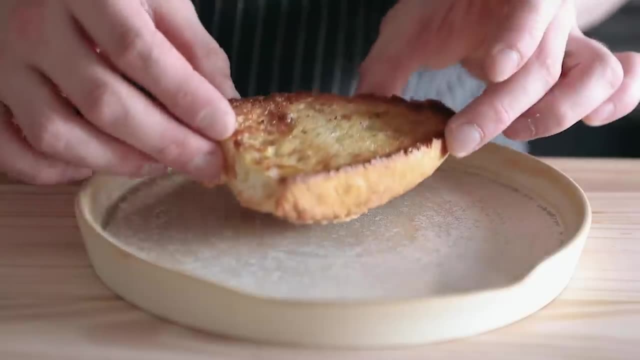 That's the beans, bro. Before the English people lose their mind, This is basically a beans on toast, but not like English beans on toast, It's just literally beans on toast. Just get a good piece of bread that you like. You can use regular toast, a French baguette like this. 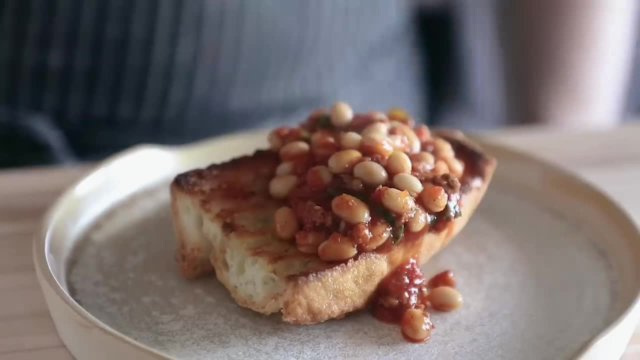 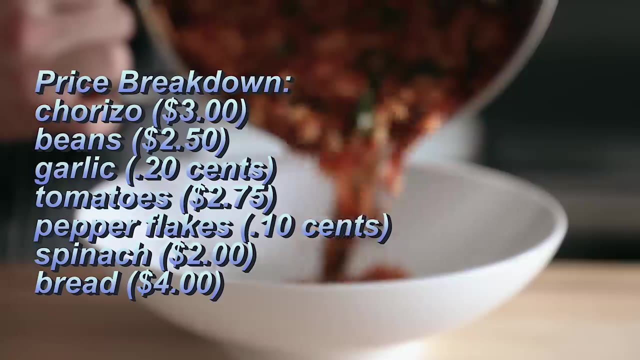 just toast it nicely, hit it with a little bit of butter and then pour this stuff on top. I also added a little bit of Parmigiano Reggiano and parsley, but that's totally optional. It's delicious without it. Okay, So here's a rough price breakdown. We've got the total cost without 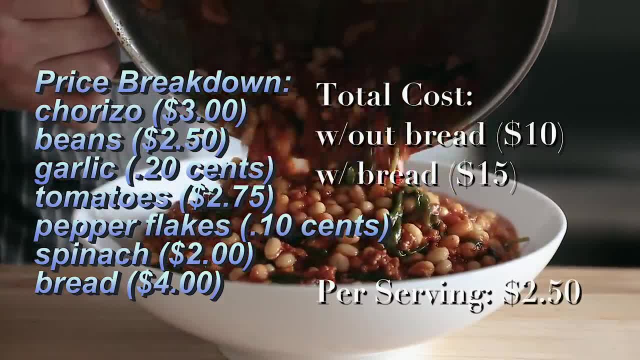 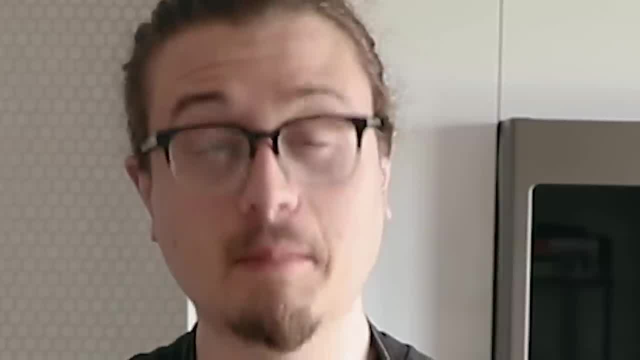 bread: $10 and 55 cents. with bread It's about $15. total cost per serving is about $2 and 50 cents with bread. It's pretty dang good for the English people who are watching. I apologize, A little Italian, some sort of uh, it's a good. 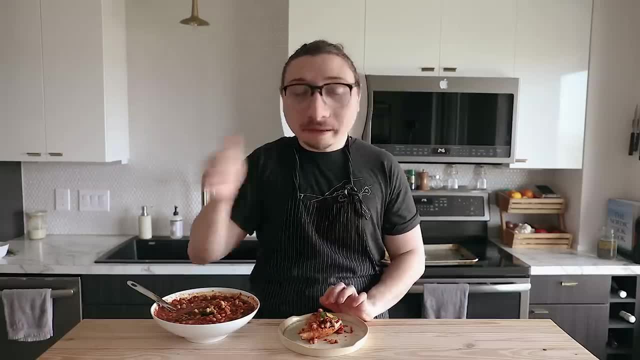 I could charge $14 for this If I wanted to West the one industry. I have a whole hell of a lot left. It doesn't have to go in this, It can go on rice. You make it, you packed it up and just put. 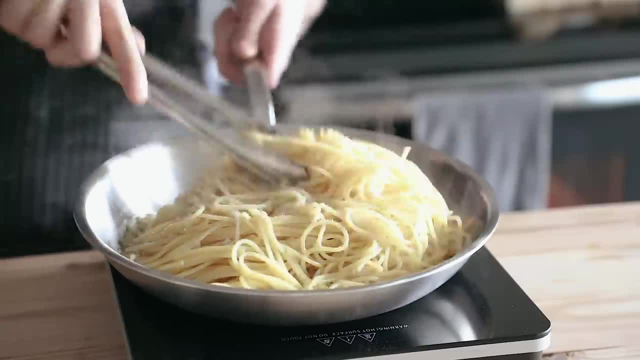 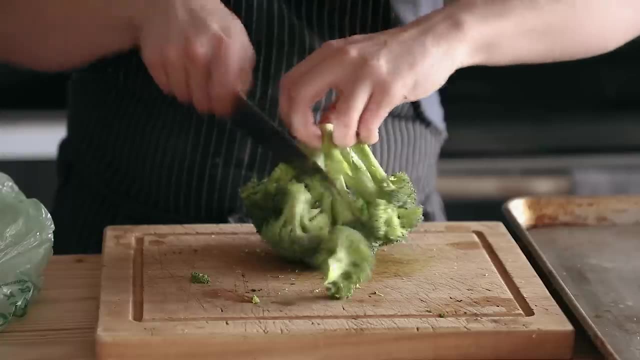 in the fridge. Now for dinner, we're going to be doing pasta Aglio e olio. Did I do that right? I hope so. Now you can eat it straight up as this, but I also cooked off some chicken breasts and roasted some vegetables. 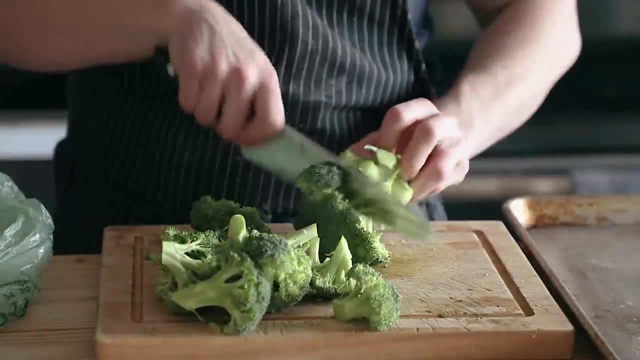 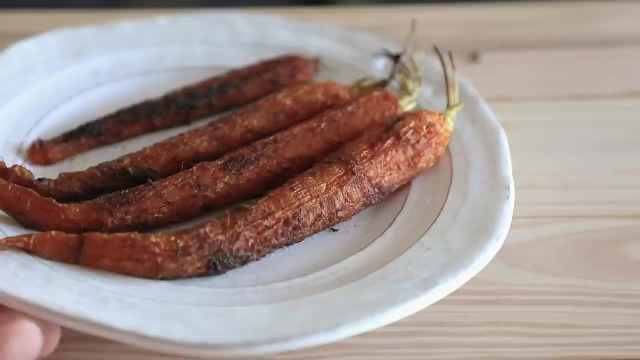 which brings me to another point. If you take a boat, little vegetables like this broccoli or these carrots, toss them with a little bit of oil, some salt pepper- You can also put spices on them- and you place them in an oven and set to about 425 Fahrenheit just until they get a little. 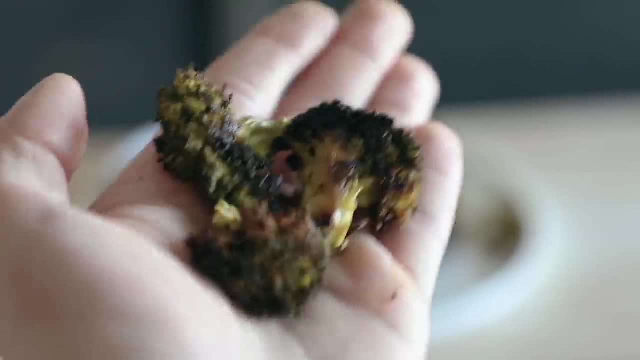 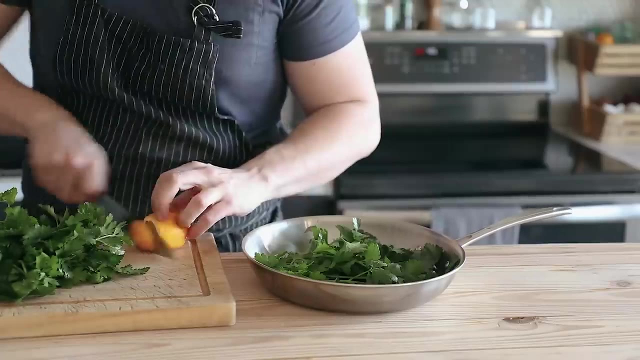 charry little soft, kind of like this. Then you can just make a bunch at a time, store them in the fridge And then you've got loads of vegetables to use and other things. but I'm off my soap box with that, Okay. So before we make our pasta, let's prepare our chicken boobies. I use bone and 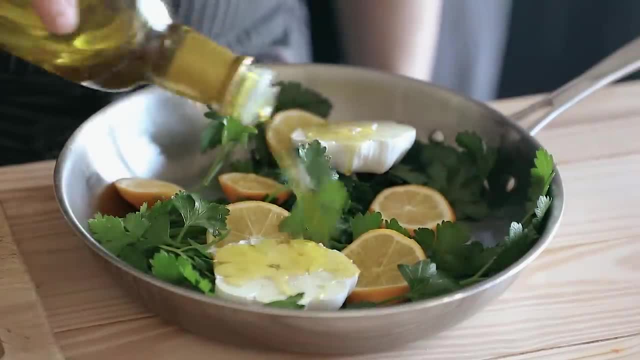 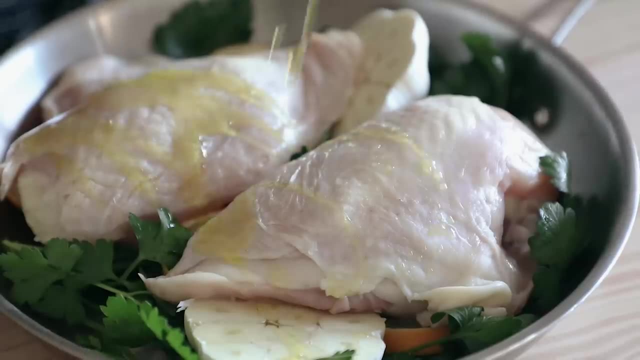 onion, split chicken breasts. You can do five, you can do 10. I just did two here. Now I did this in a stainless steel pan where I kind of like filled the bottom with herbs and lemon and all that stuff. But you can also just do it plain on a baking sheet If you have a bunch of them. 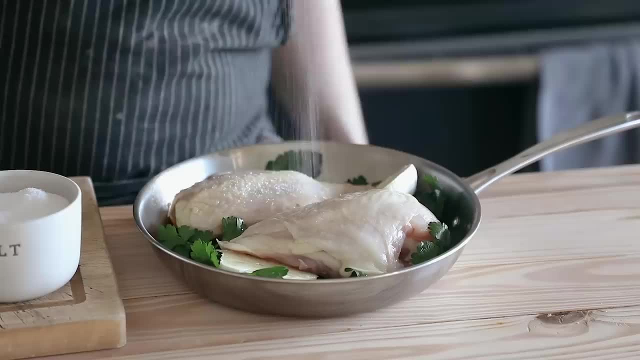 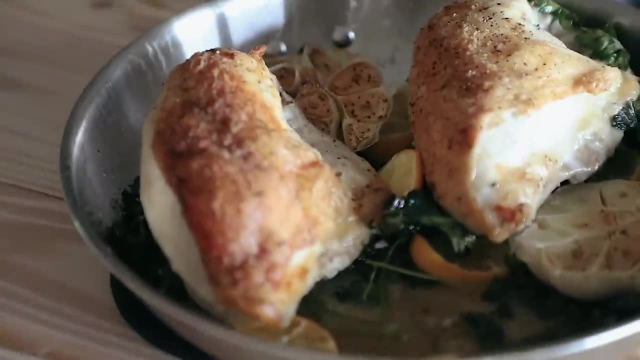 there's no problem with that. Just drizzle them with a little bit of olive oil, rub them down, season them heavily with salt and pepper and then place them in an oven set to 425 degrees Fahrenheit or 220 degrees Celsius for about 25 to 35 minutes, or until the skin is nice and crispy. 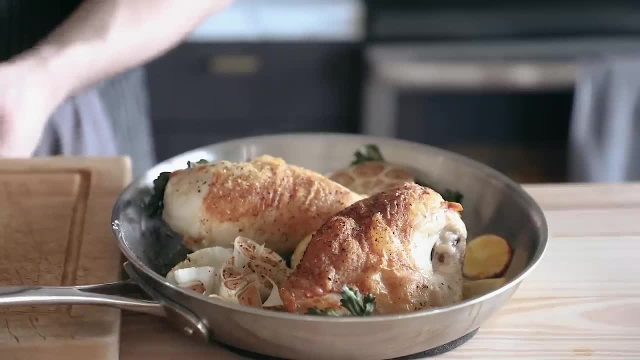 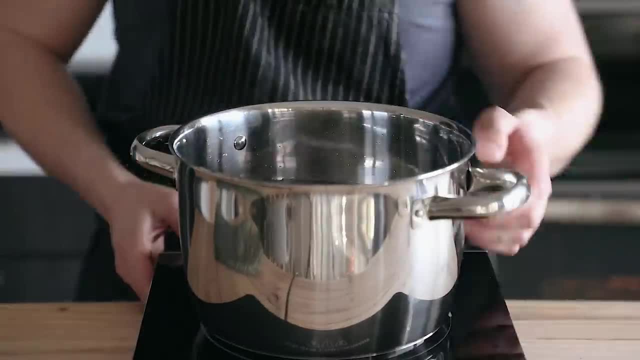 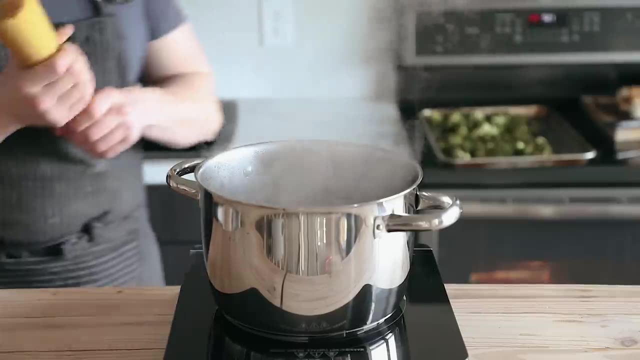 I usually pull them about five degrees early To make the pasta. bring a medium sized pot filled about three quarters of the way up with water to a boil seasoned heavily with salt. Like I want this bit salty. Once it comes to a boil, you're going to add one pound of spaghetti to it. Cook that. 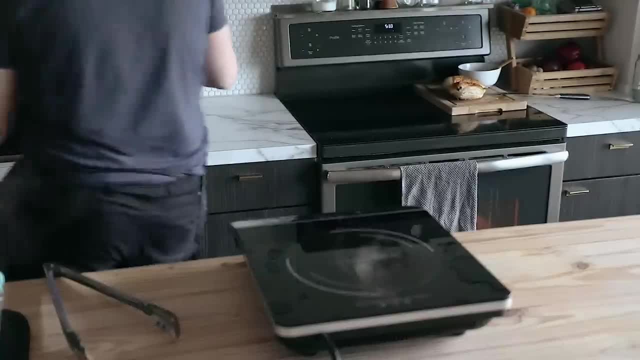 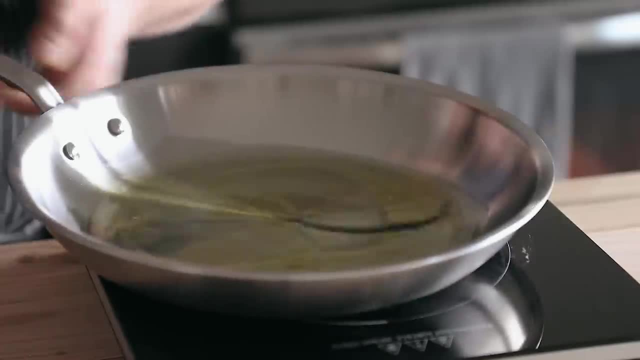 until al dente. Make sure you reserve about half a cup of the pasta water and then, well, drain your pasta. Yeah, we know how to do that. Now, separate pan. You're going to add a quarter cup plus two tablespoons of extra virgin olive oil. bring it up to heat just until it's hot. Don't get it smoky. 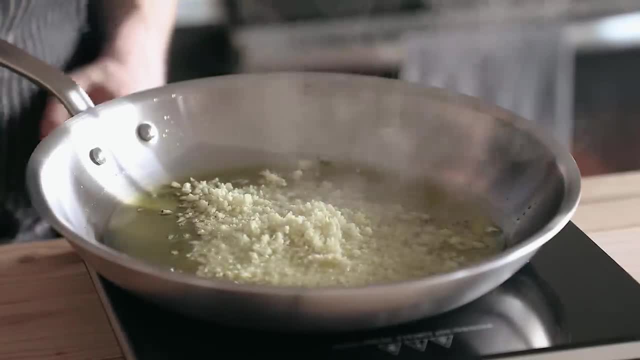 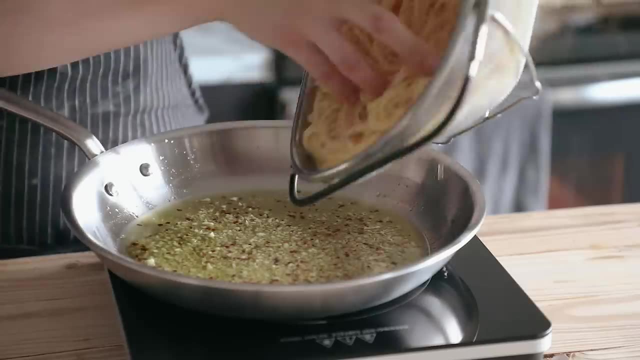 just until it's super hot. Then turn the heat off and add four cloves of finely chopped garlic along with half a teaspoon or one gram of crushed red pepper flakes. Sort a little around, let it get nice and fragrant. Then add your pasta to this pan. Toss very well to coat Adding your pasta. 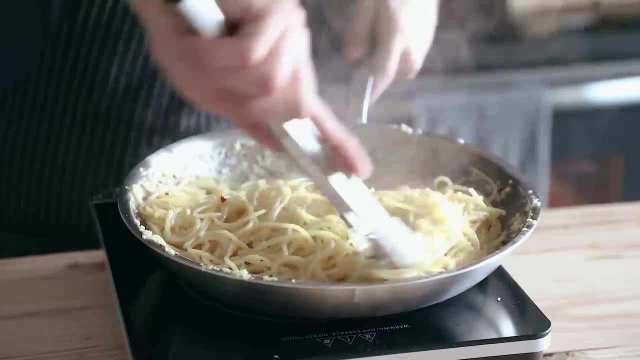 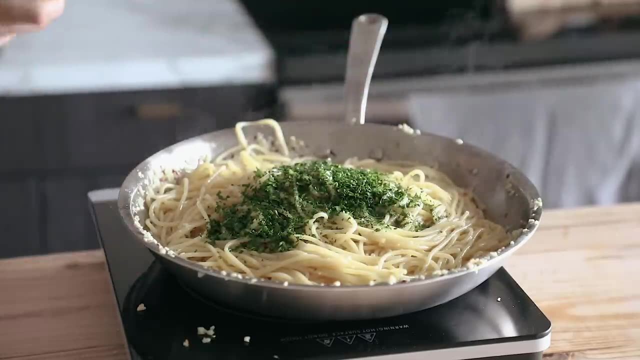 water, then toss, toss, toss. Make sure to make a humongous mess. I never get the right size pan for this, for some reason. Then adjust the salt levels and add a quarter cup or 10 grams of finely chopped parsley. Toss that together. That is the easiest pasta of all time and it's so cheap. 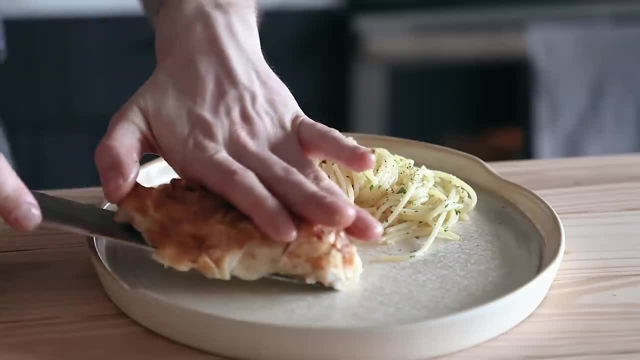 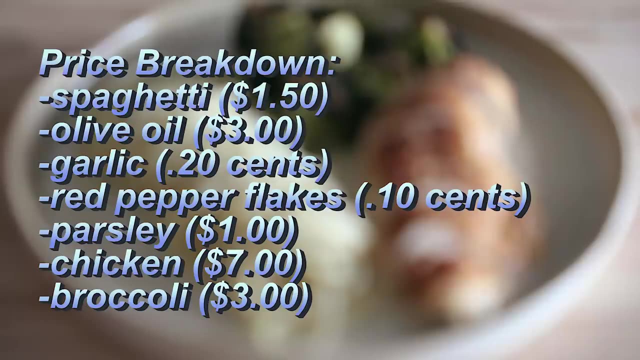 to make. Just serve that onto a plate with your chicken And your roasted vegetables. You get it, you know. And also you could just have the pasta by itself. It's incredible by itself, Okay, so here's our little price breakdown With all this put. 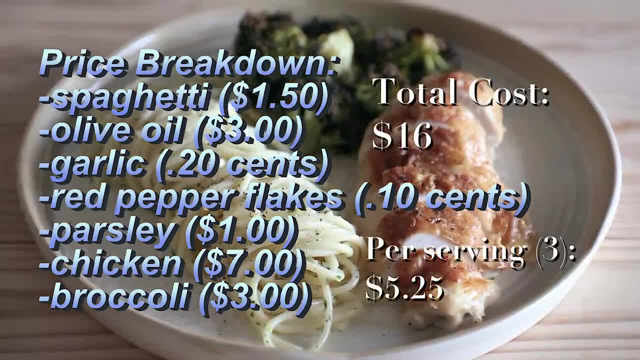 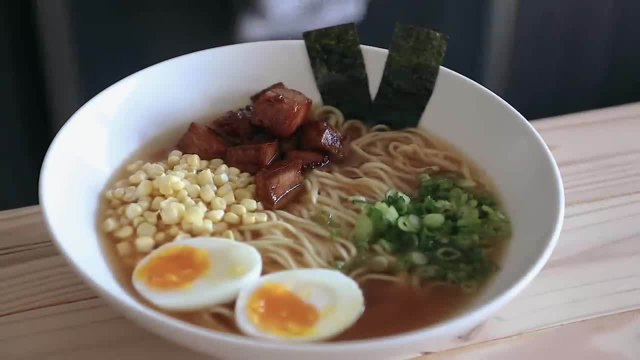 together, we got a total cost of about $16 per serving. for about three people, It's about $5.25.. Not too shabby, Okay. so it's time for bonus round, which is basically just going to be an instant ramen remake. since we're on the subject of college students a little bit, Start off by 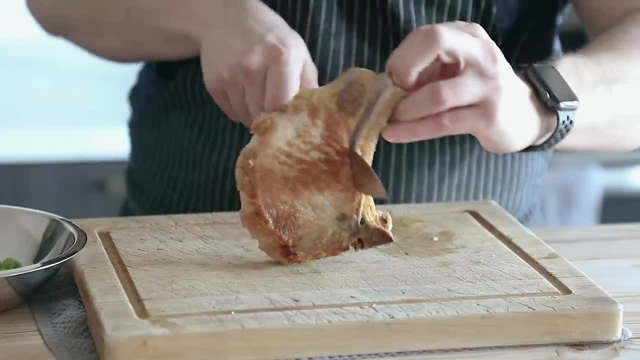 cutting some nori into strips. Thinly. slice some green onions. Cut up some protein that you might already have pre-prepped. Whatever meat, it doesn't matter. If you're making it some sort of a miso instant ramen, then I would really recommend that you cut up some corn. You. 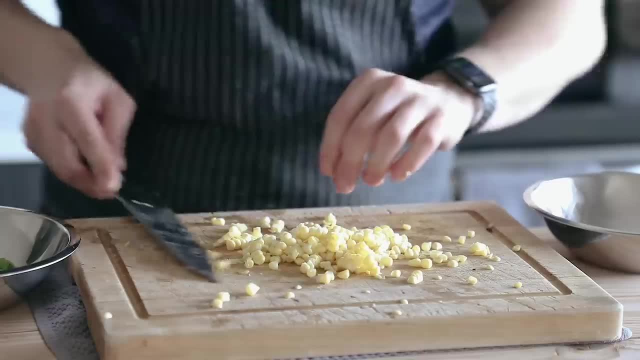 can leave it raw, You can grill it, You can char it. Honestly, I think it's great raw And I know a lot of people are going to be like ew, gross, It's really common. all right, So once you've got, 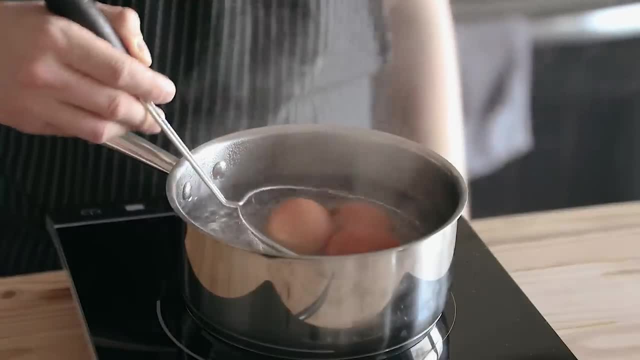 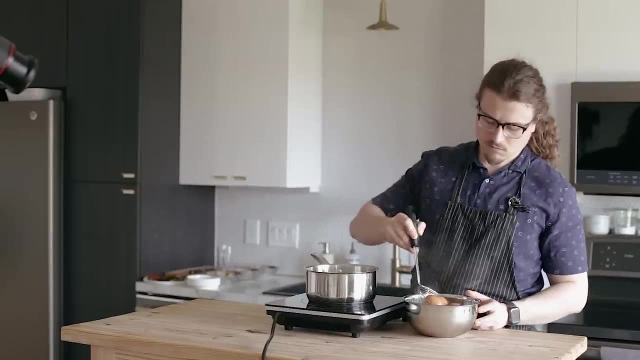 all that gathered up, let's make some soft-boiled eggs- However many you want. Just bring a small pot of water to a boil, Gently submerge your eggs and let them cook for about seven minutes. Then immediately cool them down in an ice bath until they're warm. you know about a couple minutes. 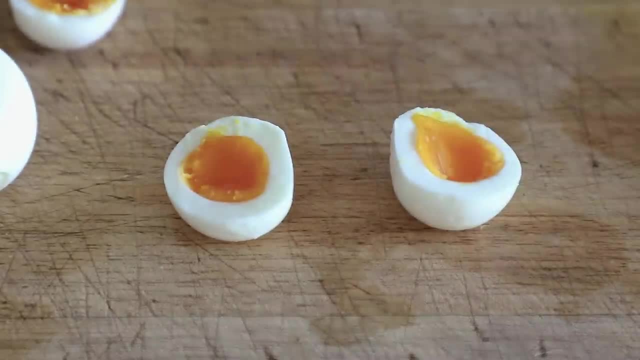 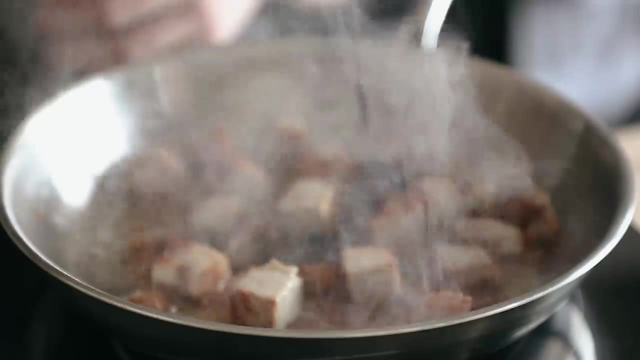 And then gently peel them And look at that. You've got a beautiful soft-boiled egg. Now for the meat. you know, you can heat it however you want. I had some leftover pork chop that I cut up. I crisped it up in a pan. I added a couple tablespoons of mirin. 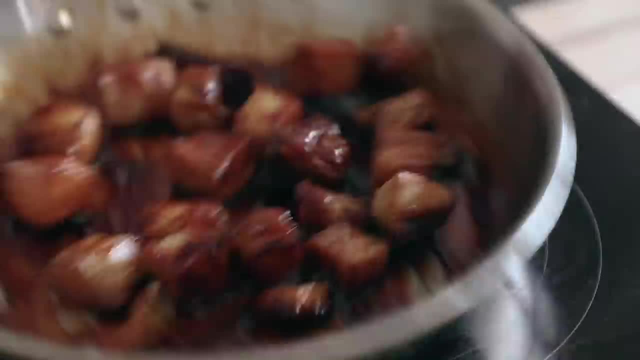 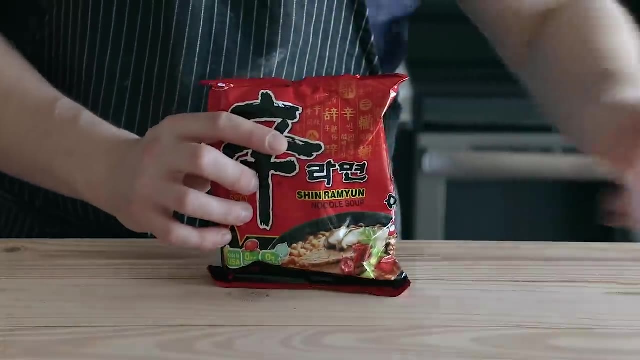 a couple tablespoons of sake and a couple tablespoons of dark soy sauce and let that reduce until we got a nice syrup to coat. Now we're ready. You just need to choose a ramen that you want. Now I've got all these different choices here. I decided to go with this, Nisen.